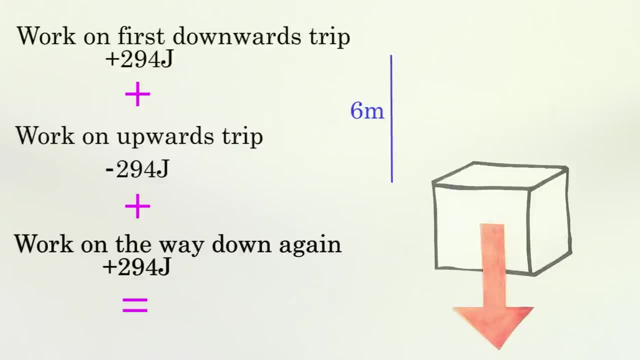 That means that the total work done on the mass from gravity is still 294 joules, just like it was when the mass was lowered only once. In other words, the work done by the gravitational force doesn't depend on the specifics of the path taken by the mass. 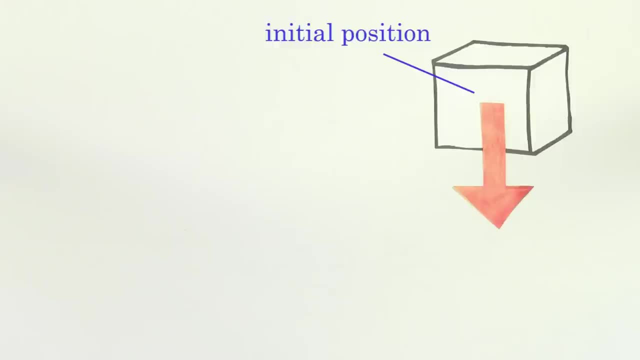 The work done by gravity only depends on the initial and final position of the mass. In fact, you could allow the mass to take any path from this initial point to the final point and the work done by gravity is still just going to be 294 joules. 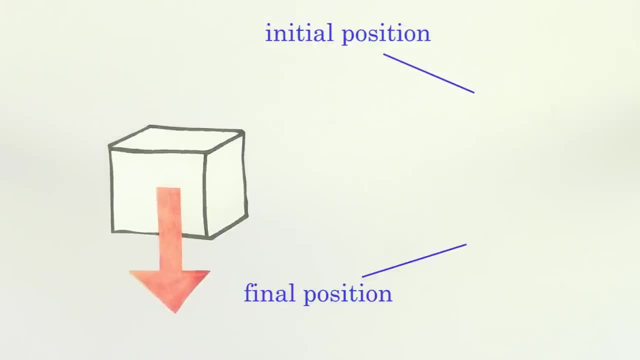 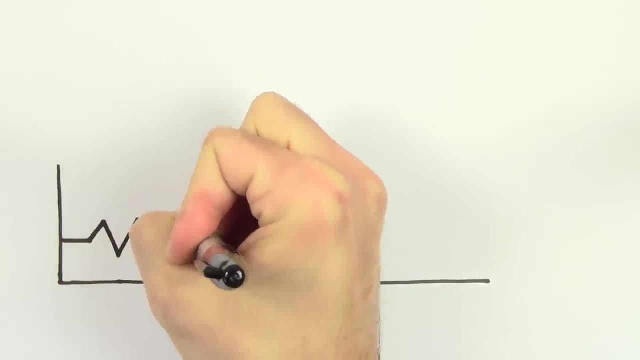 Because the work done by gravity doesn't depend on the path taken, we call gravity a conservative force. The force exerted by a spring is another example of a conservative force. The total work done on a mass by a spring does not depend on the path taken by the mass. 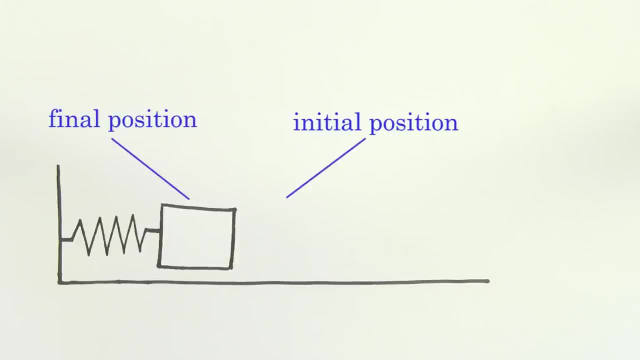 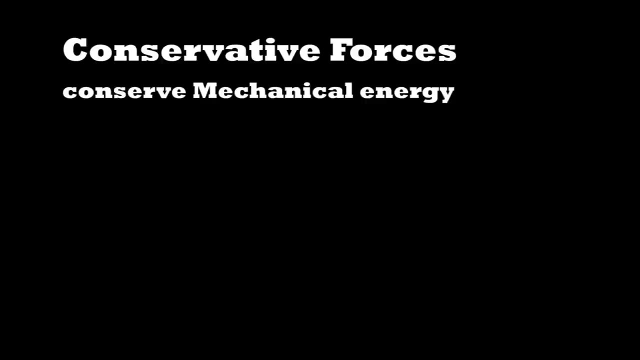 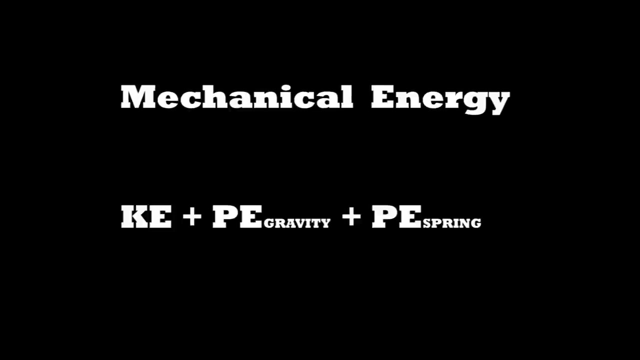 it only depends on the initial and final positions of the mass. The term conservative comes from the fact that conservative forces conserve mechanical energy, whereas non-conservative forces do not conserve mechanical energy. Mechanical energy is kinetic energy and potential energy. An example of a non-conservative force is friction. 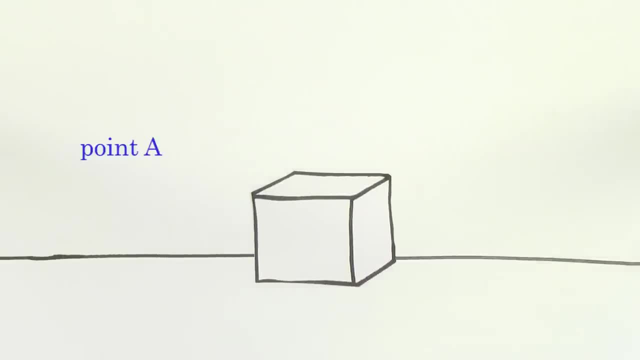 If I move a mass along a spring, moving a table from point A to point B, friction does a certain amount of negative work on the mass, which creates some thermal energy. If, instead of going straight from A to B, I make the block go from A to B, back to A, over and over again. 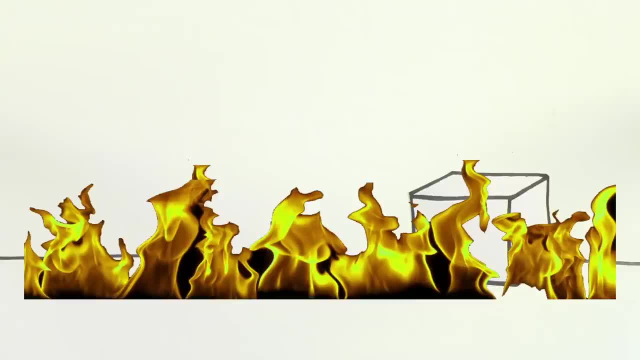 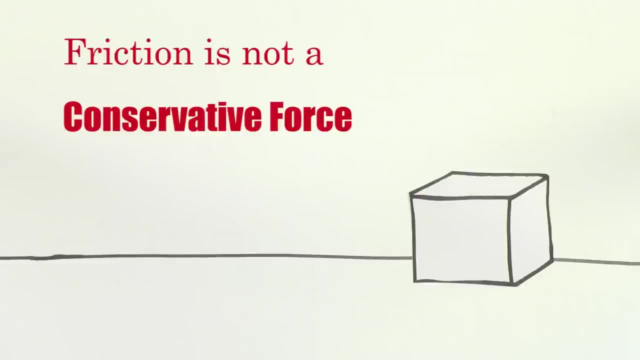 the work done by friction will become larger and larger and it'll generate more and more thermal energy, Because the work done by friction depends on the path taken. friction is not a conservative force. Similarly, air resistance is not a conservative force and the work done by air resistance depends on the specifics of the path taken. 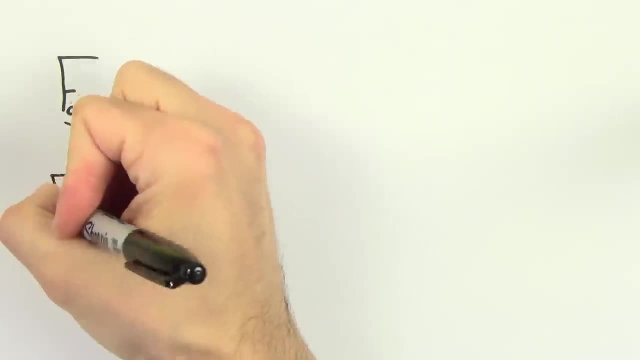 It's useful to note that if a force is conservative, you could define a potential energy for that force. That's why conservative forces like gravity and spring forces have potential energies associated with them, and non-conservative forces like friction, do not have potential energies associated with them.